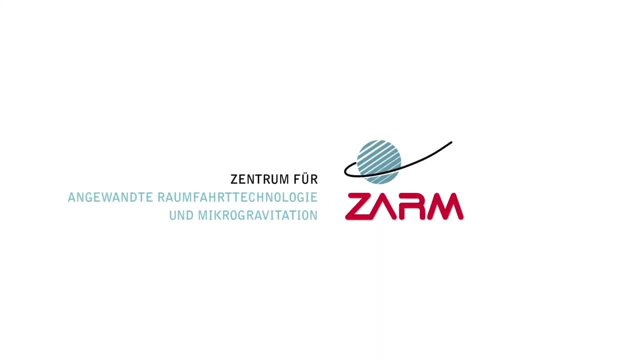 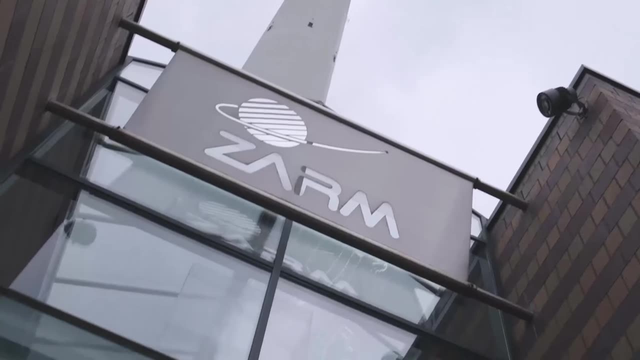 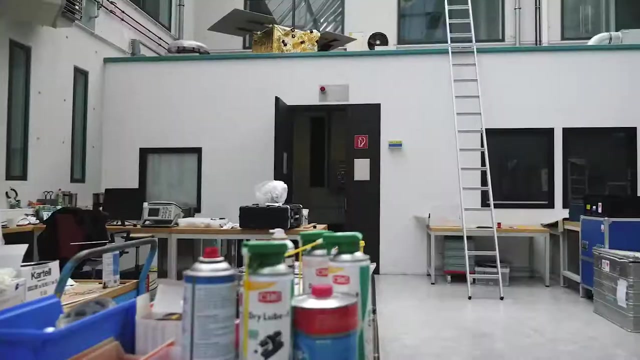 Welcome to Zahm, the center of applied space technology and microgravity. We are the operator of the biggest microgravity lab in Europe, and our customers come from all over the world to conduct their microgravity experiments here. My name is Jasmin and today we are going. 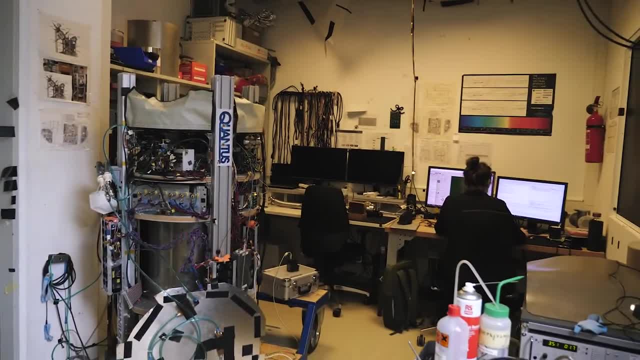 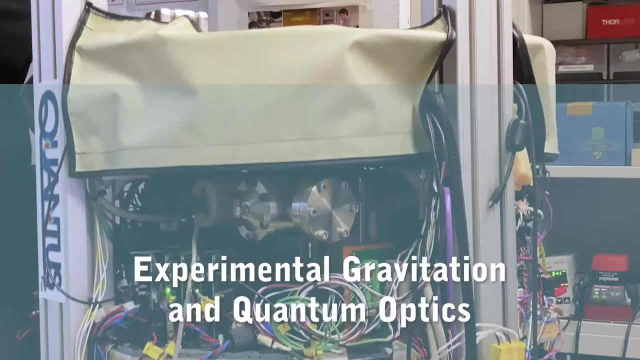 to check out the research that happens right here at Zahm, And in order to do that, we are meeting my colleague, Sven Herrmann. Hello, Sven, Hi Jasmin. Sven is heading a research group called Experimental Gravitation and Quantum Optics. Sven, tell us about your work. 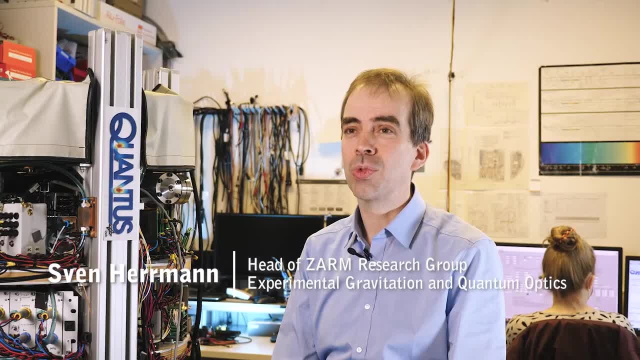 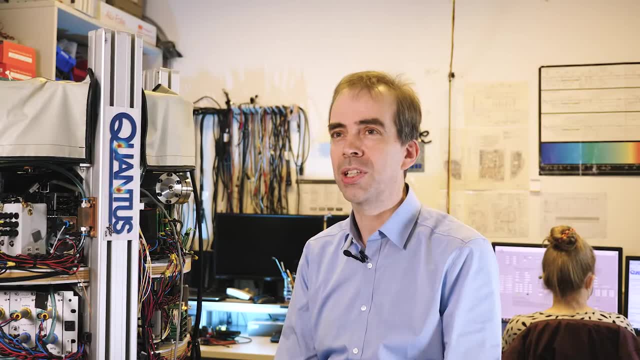 In my research group we study the physics of ultra-cold atoms and quantum gases, particularly microgravity, For example. we try to use them in tests of fundamental physics, but we're also investigating how they could be used in applications of quantum sensing. So I 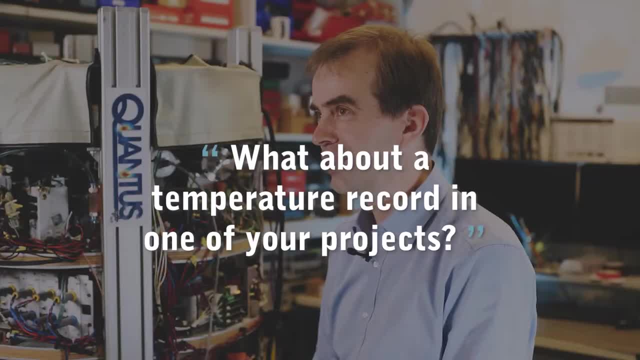 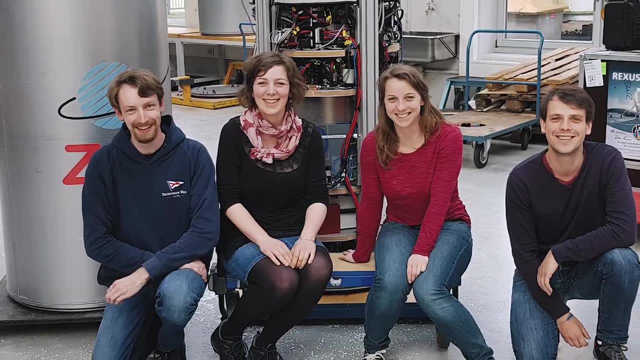 have heard that you and your team managed to reach a real-world understanding of quantum sensing. You mentioned that you have a really, really low temperature in one of your projects. What was that about? Yes, that is true. That is the QANTUS-II project. 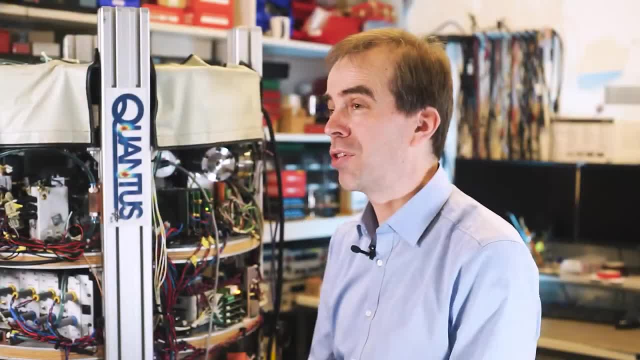 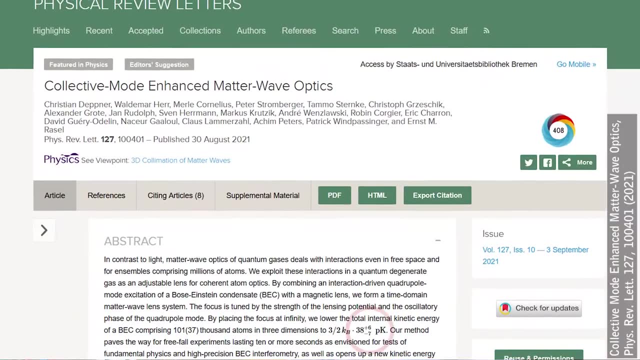 actually- and this is a collaborative project we have with a couple of other universities- And in this experiment we obtained a record temperature of 38 picocalvins here in the drop tower, And what we are talking about here is, then, really just a tiny ensemble. 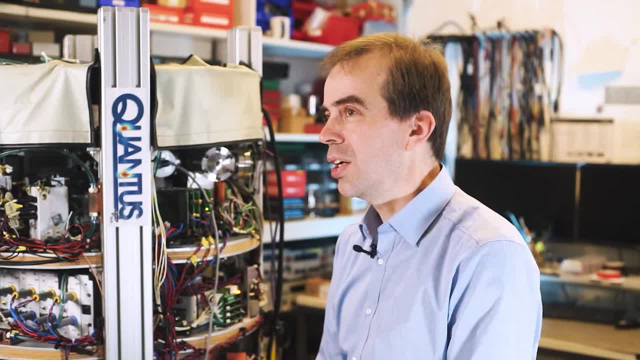 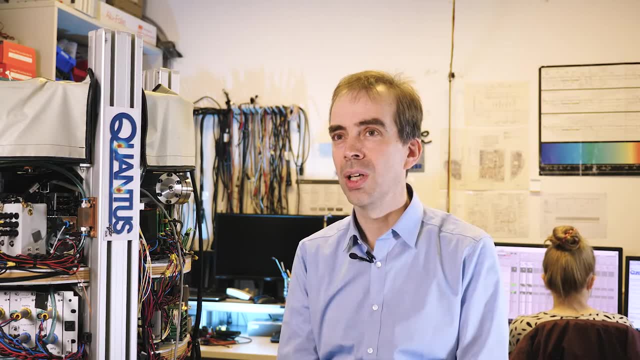 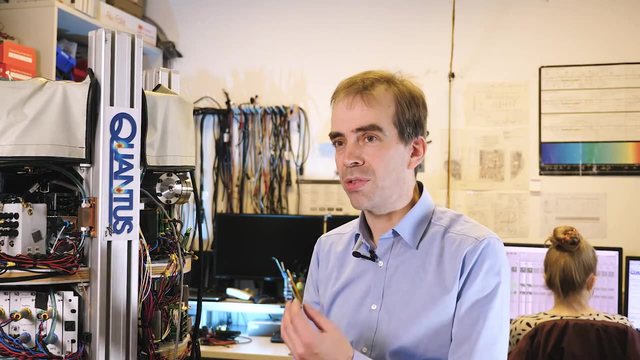 a tiny cloud of atoms, about 100,000 rubidium atoms- that we cool down. That means that all these These atoms go to one ground state, the so-called Bose-Einstein condensate, and in that state they form a coherent metal wave. Now, this was actually only a byproduct to achieve this. 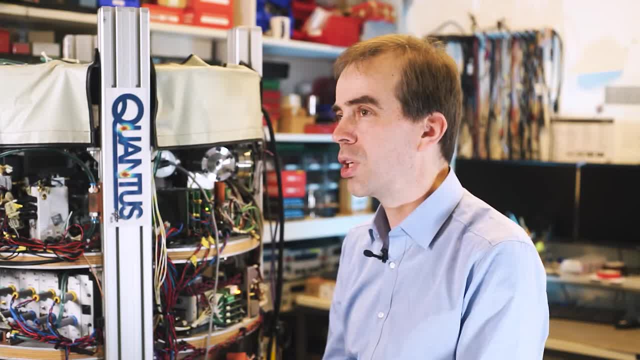 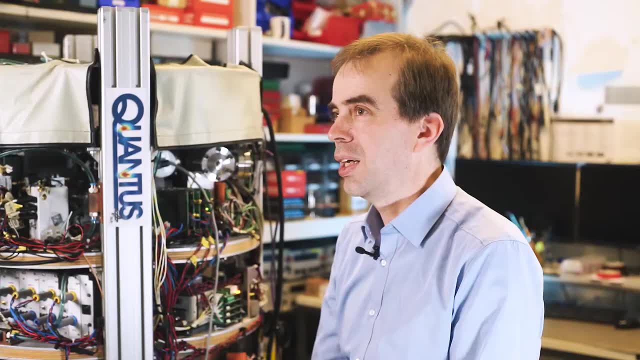 very, very cold temperature, because what we're interested in is to really slow down the atoms so that this tiny cloud of atoms does not expand too much when we use it in our interferometer, in the drop tower. And slowing down means really cooling it down to this very low temperature. 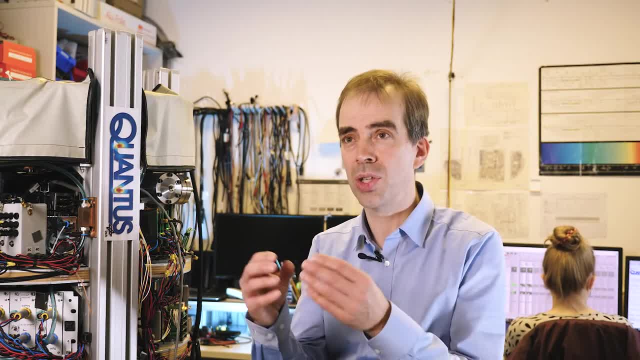 The 38 picocalvins means that on average, the atoms in the drop tower are about 100 micrometers per second. So the atoms in this cloud move with only 50 micrometers per second or so, And that's what we are actually interested in. 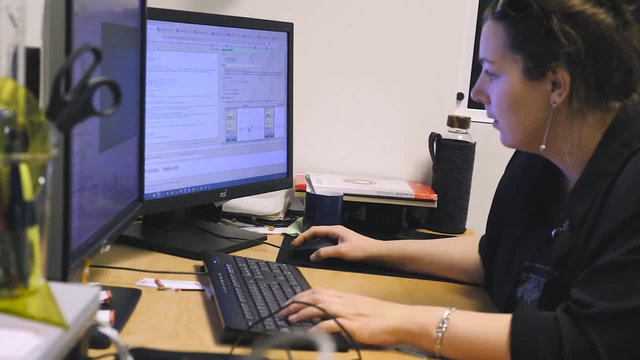 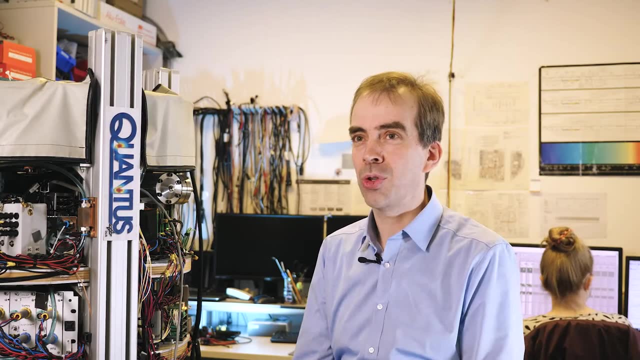 So it's about the state of the atoms, not so much about the temperature. But what is a Bose-Einstein condensate actually? Imagine you have a gas at room temperature, just like the surrounding air. here All the particles at room temperature. they move at relatively high speeds, something in the order. 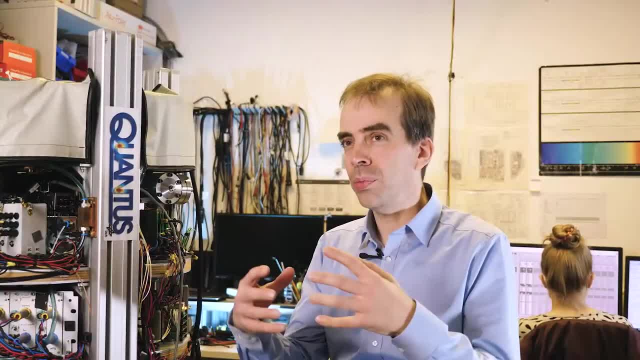 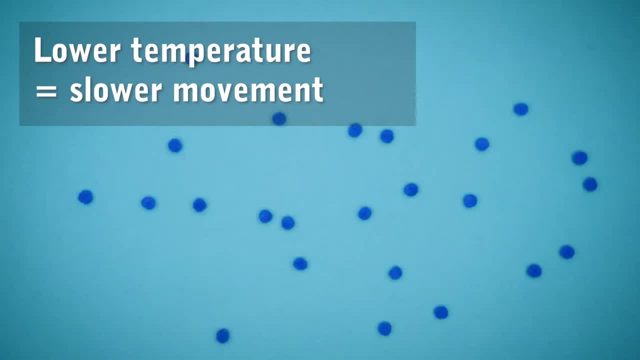 of 300 meters per second. Now, if you cool this gas down, it essentially means you will slow down the movement of the gas. It will slow down the movement of the gas And that's the movement of the atoms. Now you can imagine that all these atoms, all these particles, 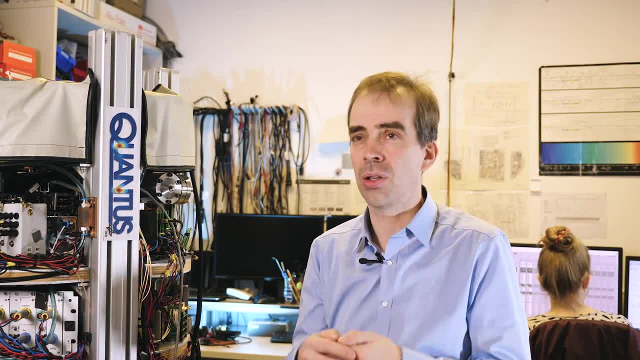 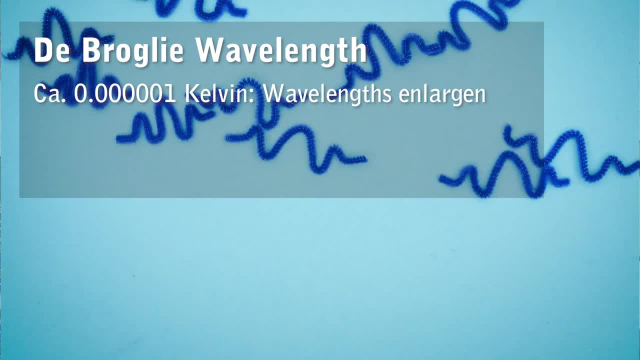 they have a quantum mechanical wavelength attached to them. That's the so-called de Broglie wavelength, And this is a function of temperature. The colder you get, the larger this de Broglie wavelength will get, And then all these increasing quantum wave packets, let's say, will overlap. 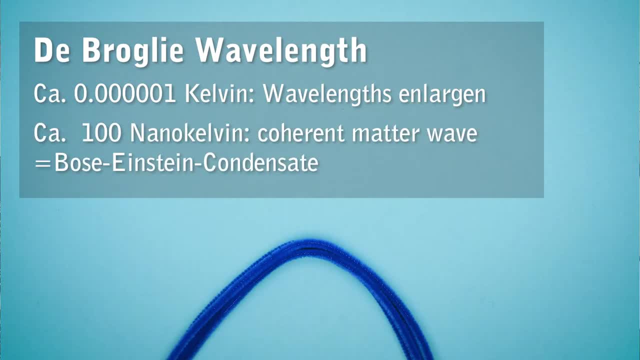 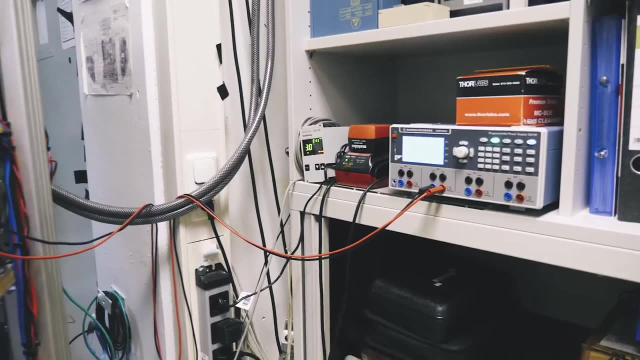 and will form a coherent metal wave. And that's when we arrive at the Bose-Einstein condensate at the level of something like 100 nanokelvins in temperature. Okay, That sounds kind of technically demanding. How do you do that? 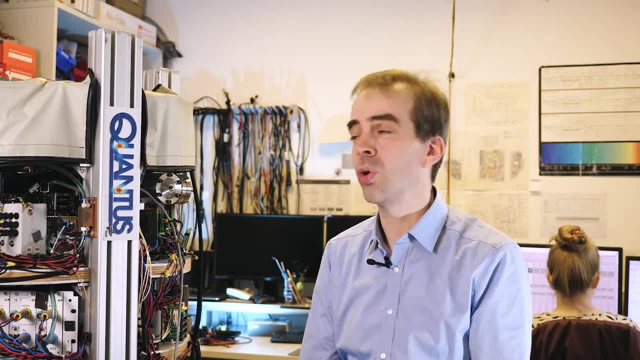 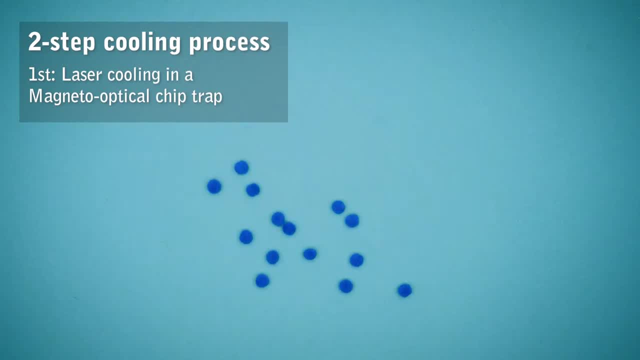 So to arrive at these really low temperatures, what we usually do, what we do in this experiment, is we use a two-step cooling process. basically, The first step is laser cooling in a so-called magneto-optical chip trap. So that's a combination of lasers and magnetic potentials where we 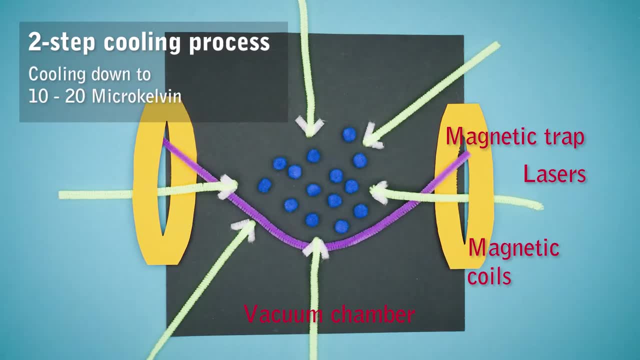 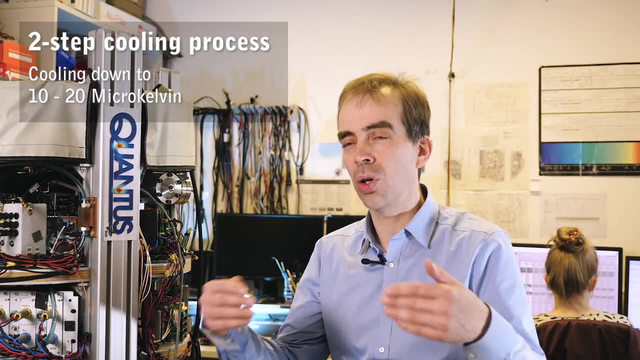 cool down to something on the order of 10,, 20 microkelvins, about 10 to the 8 atoms. And we cannot go any further if we use lasers, because we always have the recoil of the photons with the atoms. that will prevent us from getting any lower. So to go down to the Bose-Einstein, 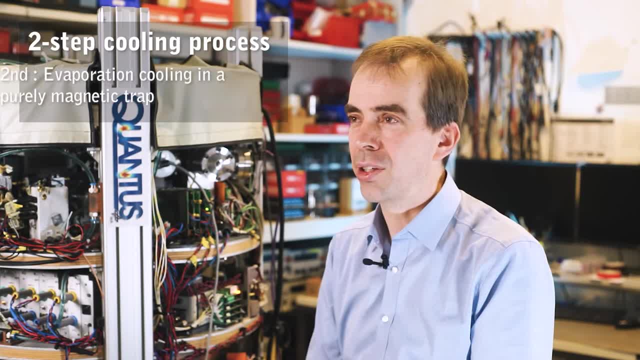 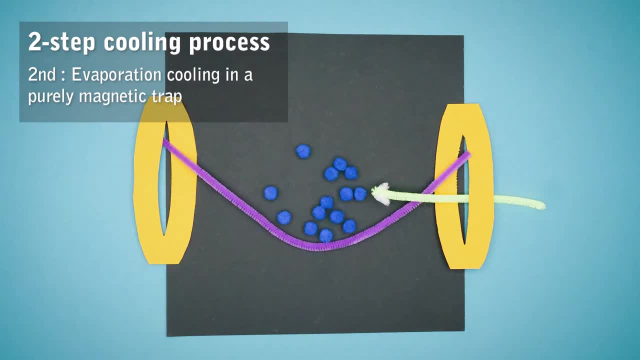 condensate at 100 nanokelvins. we use evaporation cooling as a second step, And that means we load all these atoms then into a purely magnetic trap on our atom chip And then we will evaporate the hot atoms out of this trap so that only the cold atoms remain and re-thermalize And 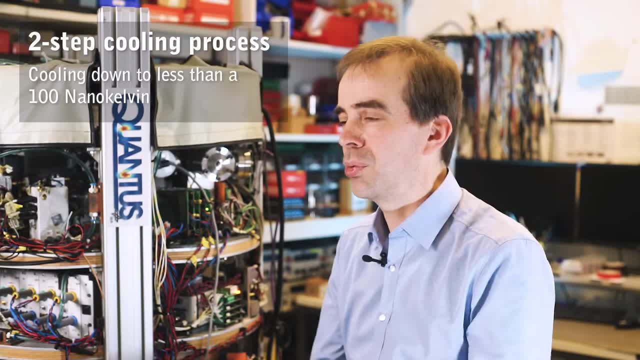 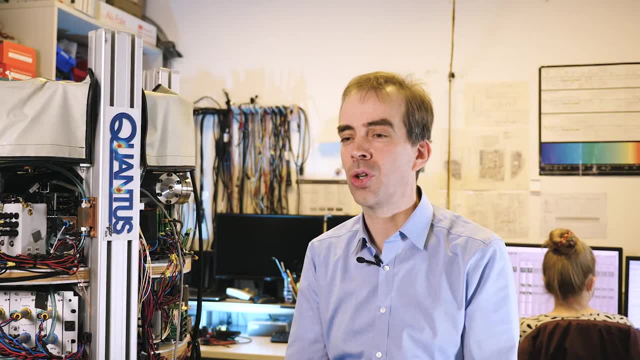 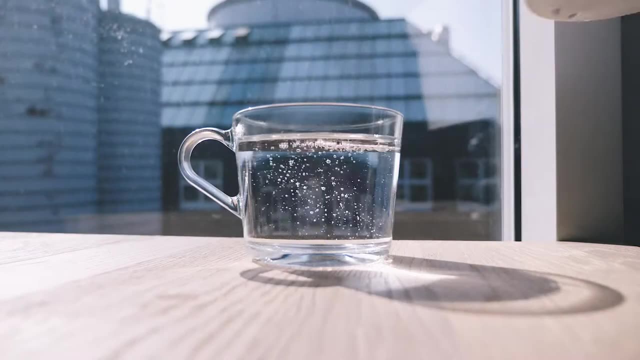 that's it, And with that we lose a lot of atoms, but we also reduce the temperature by orders of magnitude. And it's kind of comparable in principle, like the evaporation cooling that takes place in your coffee cup here, where you also have the hot coffee atoms leaving. 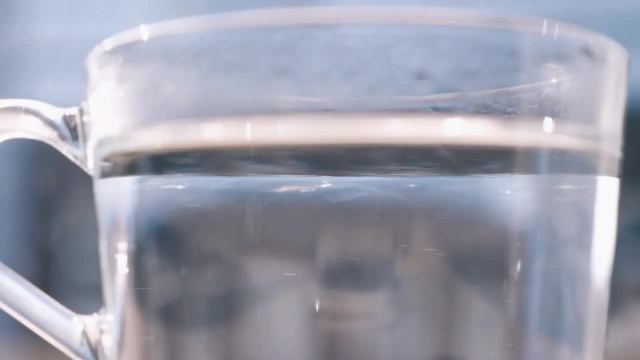 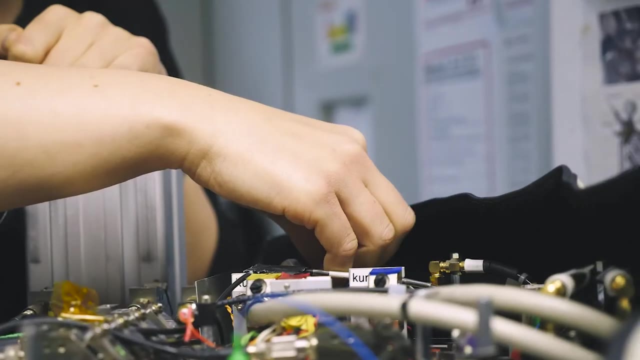 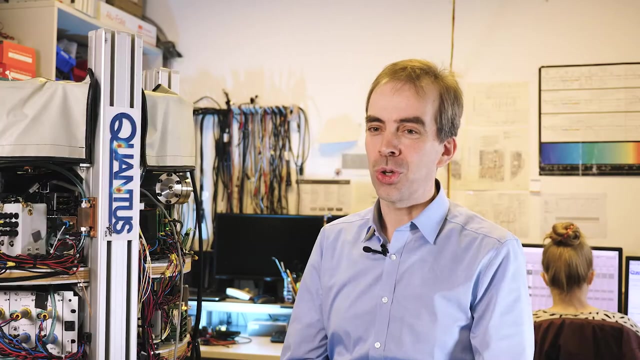 the cup and the rest of the coffee settles down at a lower temperature. Just here we do it much more efficiently and much quicker. Ah, cool. But as you and your team put all of this into one of our drop capsules, I guess the weightlessness is true. 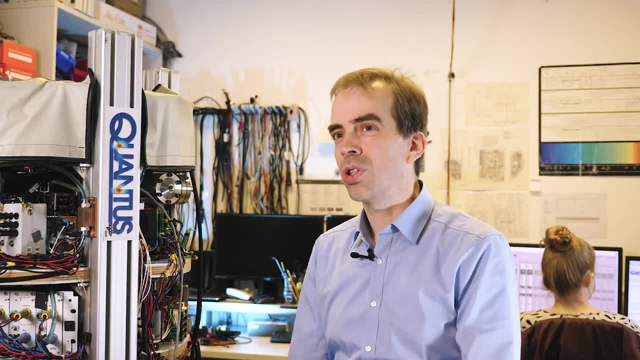 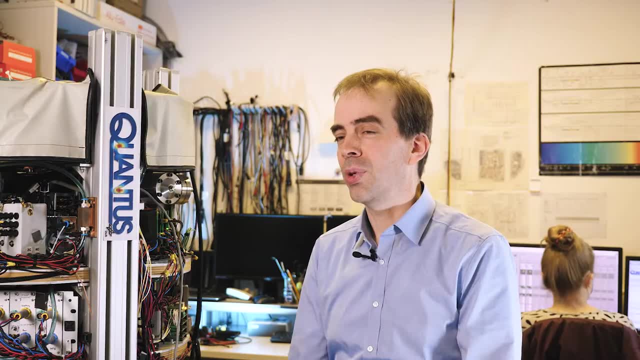 So the Bose-Einstein condensates I just described, we want to use them in metal wave interferometers. And the sensitivity of these metal wave interferometers increases a lot the more time the atoms can spend in this metal wave interferometer. Now, in the metal wave interferometer we cannot. 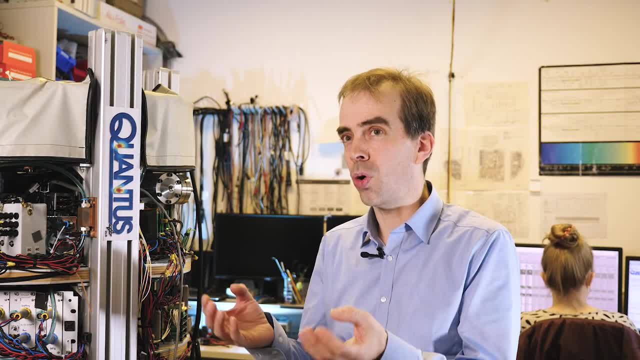 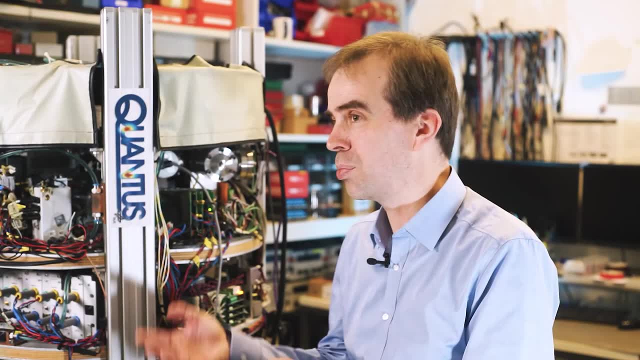 suspend the atoms. We cannot hold them. We have to let them freely fall, And that limits the time they spend in the interferometer In an apparatus here in the laboratory. it's just 200 milliseconds or something, And that's why we set up everything in a drop capsule. 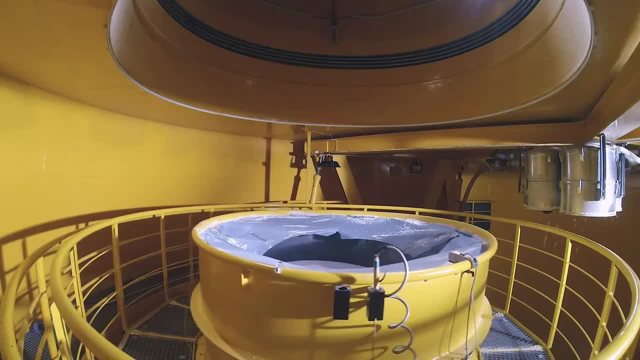 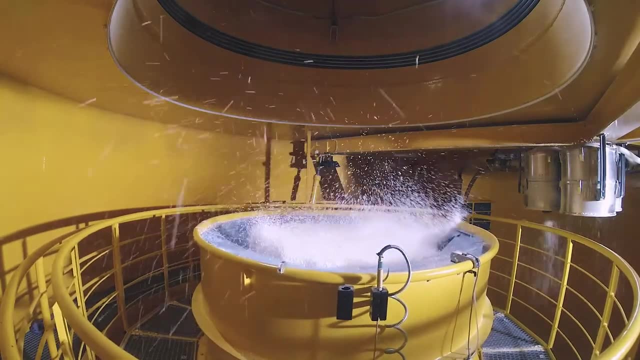 and we can go then to the catapult, to the drop tower, and we can increase this free fall time up to 9.3 seconds And that tremendously can increase the sensitivity of these instruments, particularly since the sensitivity scales quadratically with the free fall time. 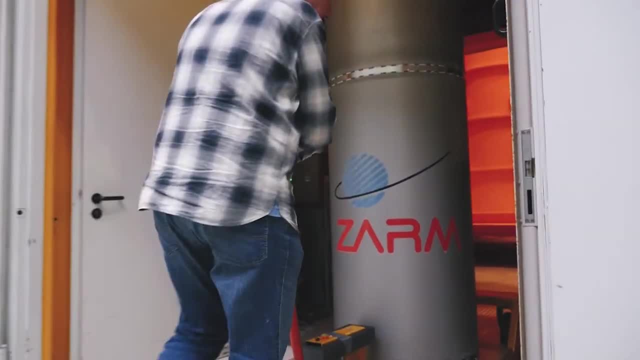 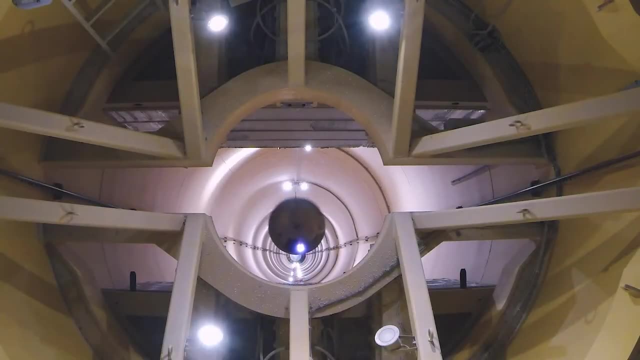 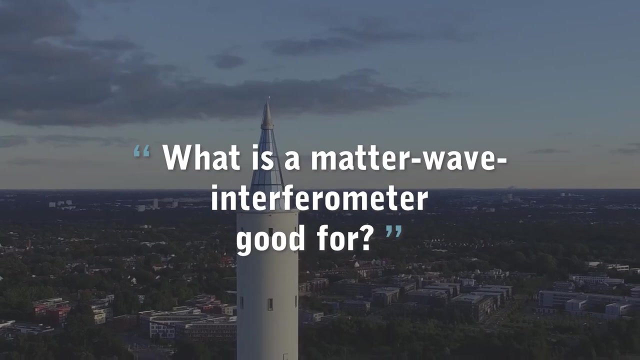 Okay. so if I understand you correctly, in normal gravity the atoms would just fall to the ground shortly after you turned off the temperature, But not in weightlessness, which is why you can observe the Bose-Einstein condensate for much longer Still. I am asking myself: what are they good for in the end? 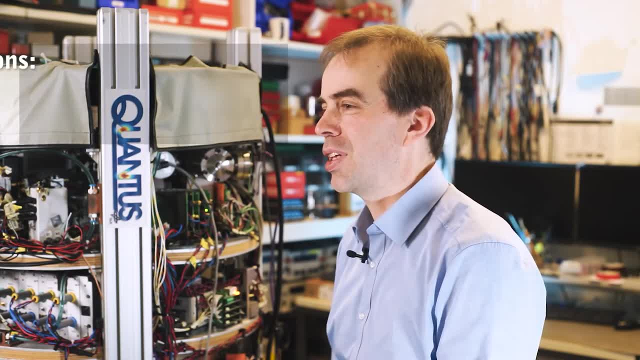 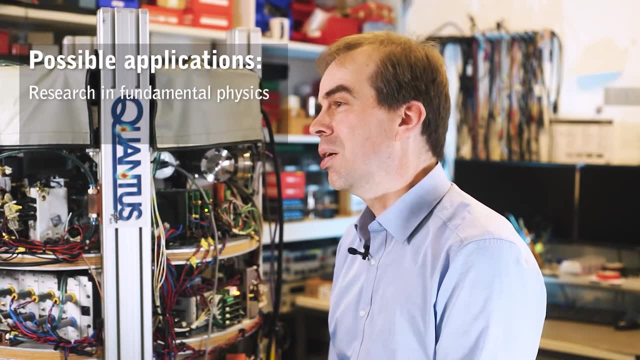 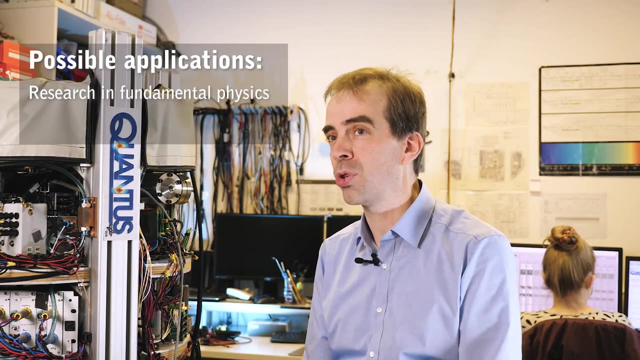 Yeah, these metal wave interferometers, they have a lot of interesting applications. So one of our main motivations is doing research in fundamental physics, But there's also some recent proposals, actually, or investigations that look at applications in earth observation and geodesy. These metal waves, they are sensitive to gravity and that means you. 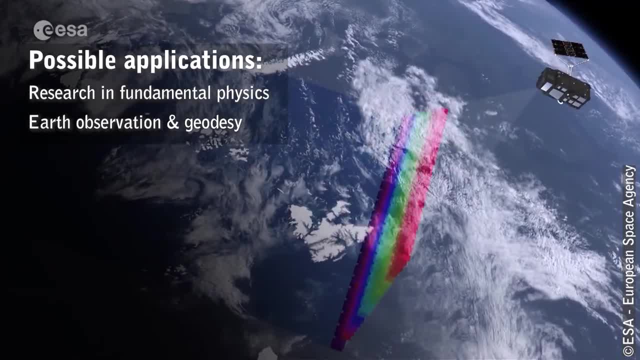 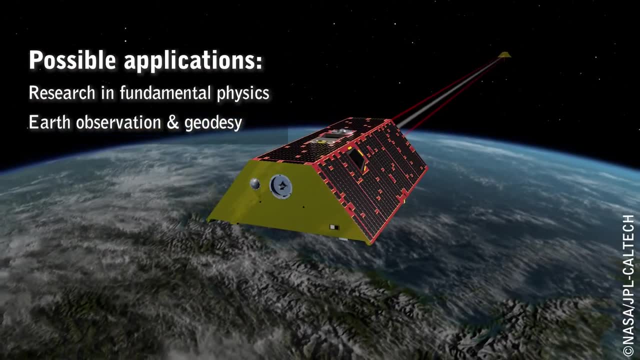 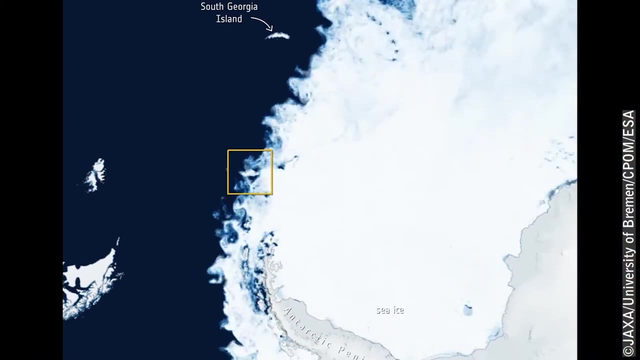 can detect really tiny variations in earth's gravity field, And this you can use in mobile devices in exploration, but also in satellite missions that do earth observation And that, of course, then can help to monitor the consequences of climate change, the melting of glaciers.